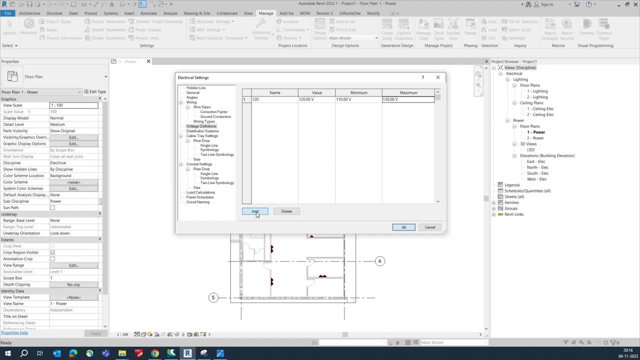 uh, 130. okay, so that was set up. and another one: i need to assign 208, okay, for example, here also to 208. minimum i can give 200 and maximum i can give 220. so like that we need to set all the voltage definition first. 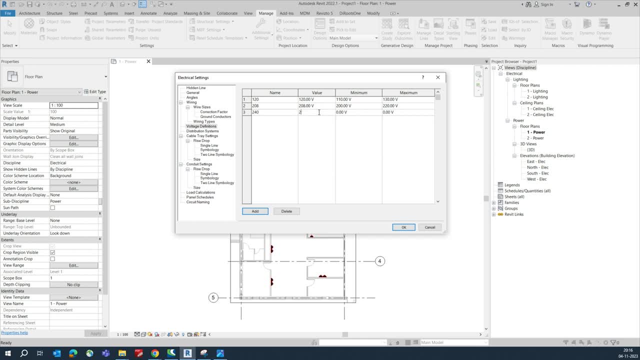 next is 240, and next this one 240, and this one is 220 and another one is: we can say like 250, the maximum, okay. so next one we need to set like 277, 277 and the minimum is 260 and the maximum is 280, okay, and next one we need to add it, okay. for example, 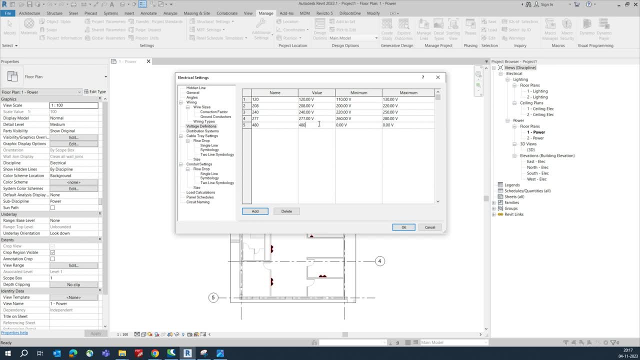 480. i need to add it: okay, 480, then minimum 460, maximum is 490.. so once you set up this one voltage definition so you can add it to maximum whatever as per your standards, you can add it to everything, then go to distribution system. then what we need to do here also, we need to add: 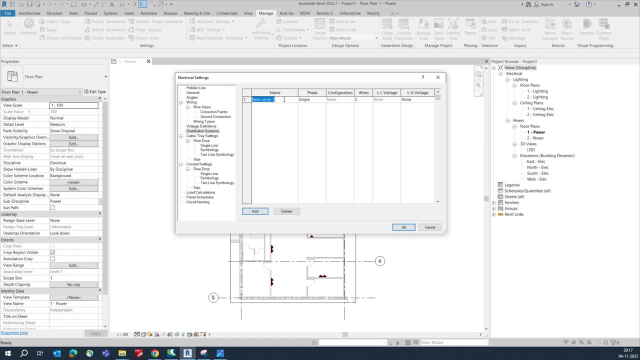 all the uh, the distribution system over here, okay. so, for example, first i will say like two, note eight, okay, um, and this one is, phase is three. and wires we can say like four, and uh, this one we can say 208, and this one we can say like 120, another one we need to add it: uh, 120, 2, 40, okay, so that one is. 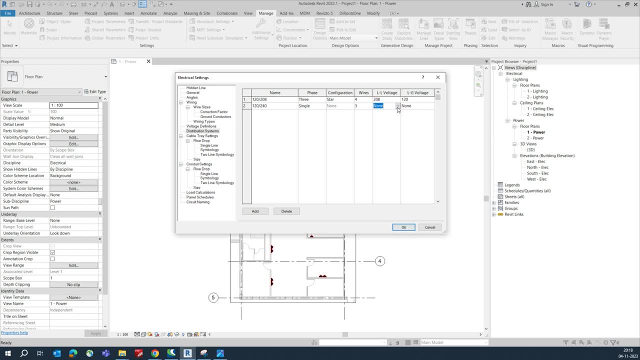 single phase, so we can say this one three, and here we can say 240, and here you can say like 120, okay. another one is, uh, 480, we need to add it, okay. so, for example, this variety is 277, okay. and three phase, and here we can give like four, and this one we can say like 480 and this one we just need to. 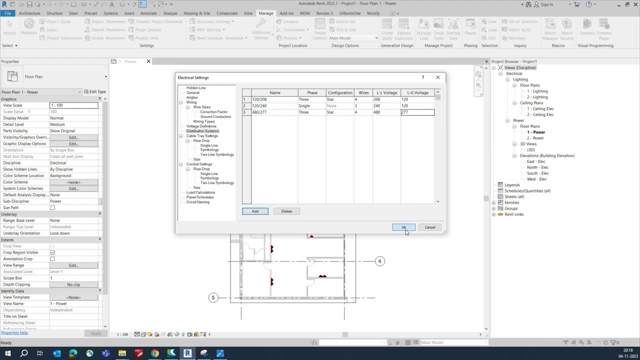 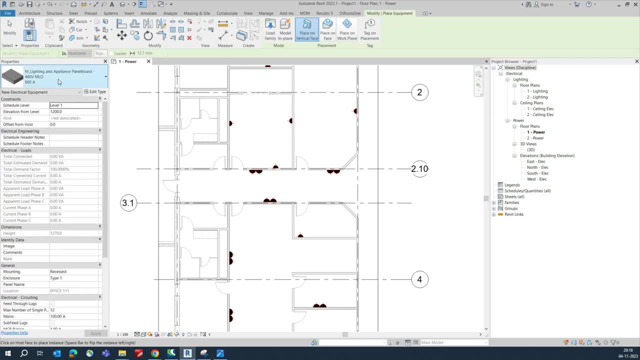 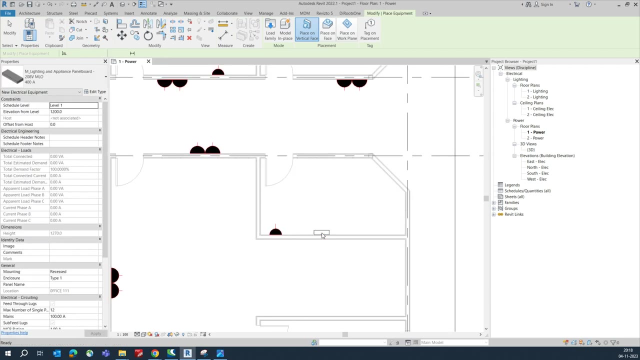 give a 227. so once, once that's set up, just click ok. then what we need to do? we just go to system tab and go to electrical equipments and we can place a db from here. okay, for example, i'm placing one db over here. okay, if you select this one, so the distribution system will be showing over here. 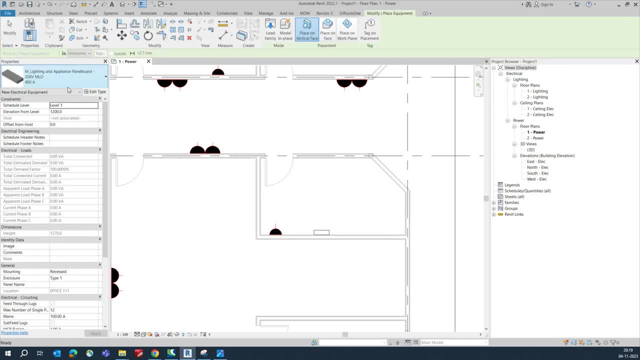 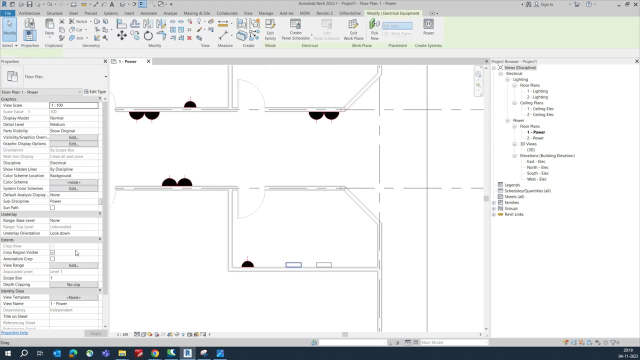 and another one. i need to place another db, uh hello, for example, this one, uh 400 amps. okay, so i'm just placing over here, so it this will be. once you selected then then the distribution system will be showing over. so we need to give a circuit, okay, so we can give the name of the panel also. so, for example, this: 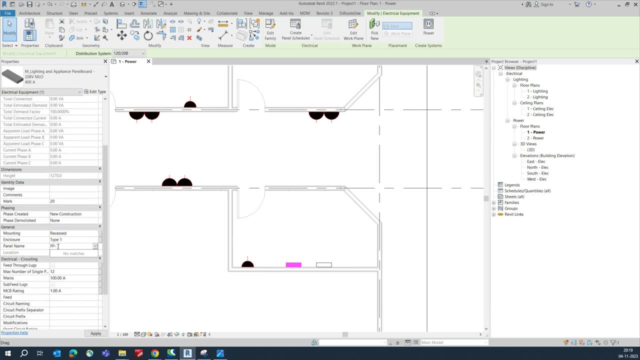 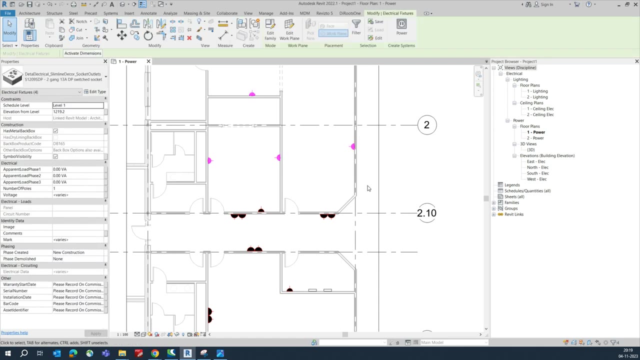 panel name is pp dash one. okay, so this just say: this one is pp dash one and this one is pp dash two. okay, so some circuit i need to connect to for this panel, so for example, this four, i just select this four- give a power. okay, then we can say like this one: okay, click ok. 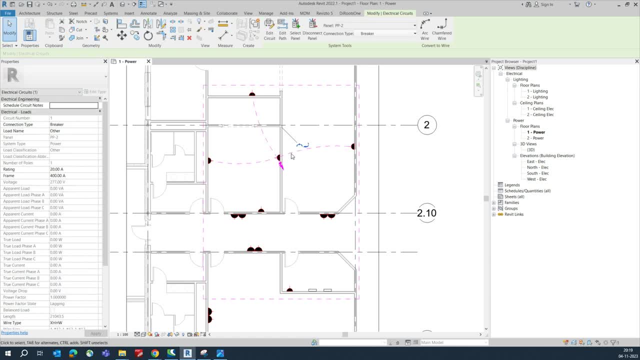 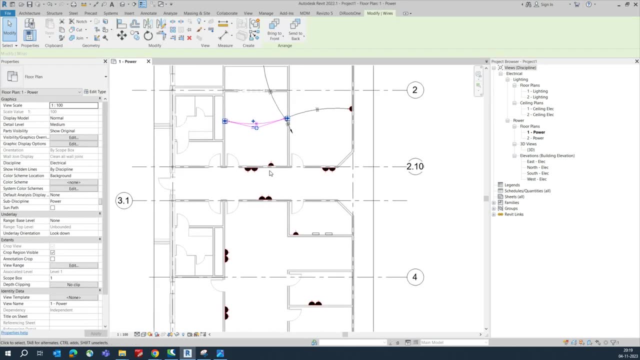 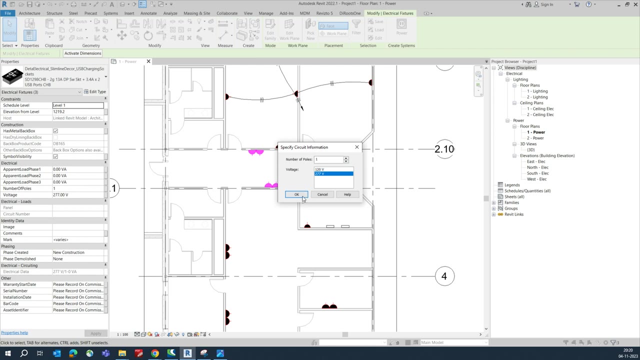 and select the panel. okay, so i'm selecting this one, so it will connect it to uh, this panel. okay, like this. you can see this: uh wires already connected to the panel. okay, for same thing. you can. you need to connect this three to here. just click that one and select this one and click ok and select the panel pp2. 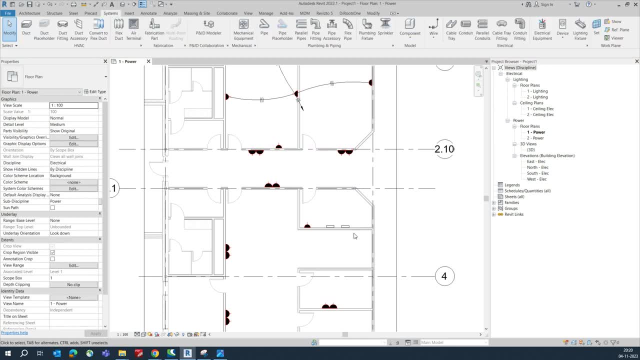 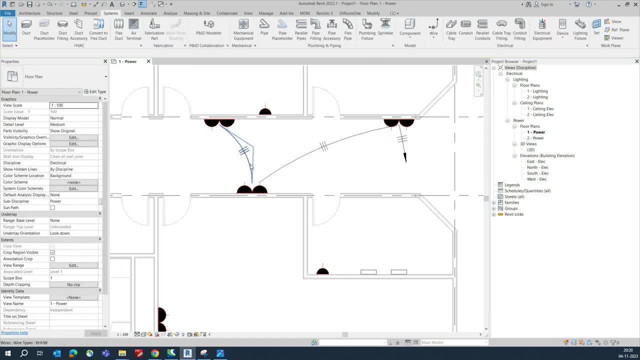 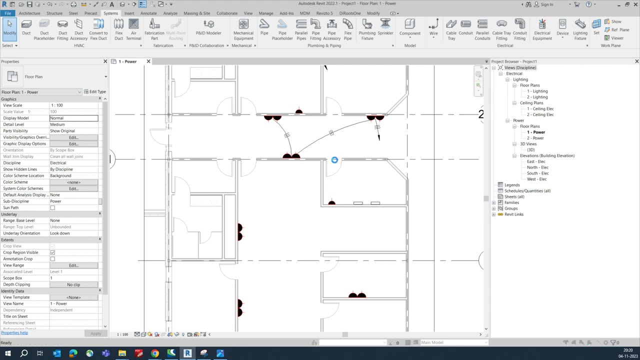 and select the panel. so, uh, sorry, uh that that that will be. that will be connected. okay, just selected. so this will be connected to this, this, that panel. okay, so you can adjust the wire like that and you can change the wire size also. type VV and go to wire. 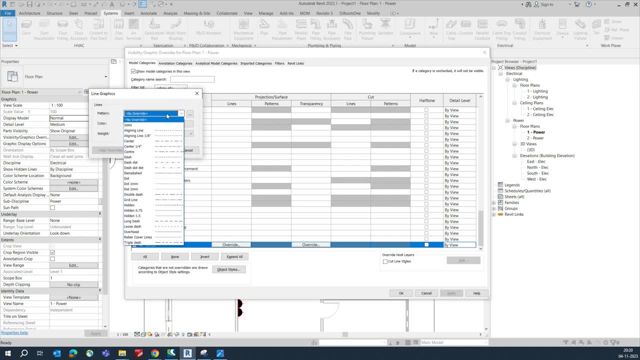 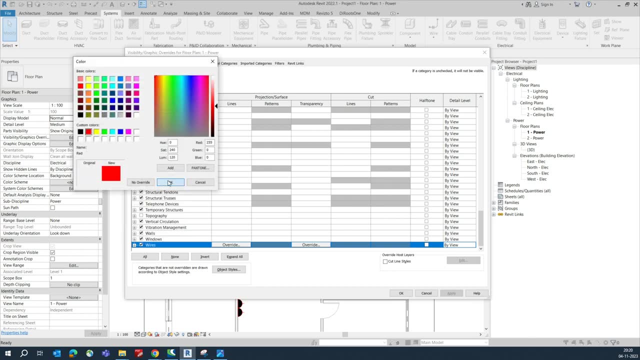 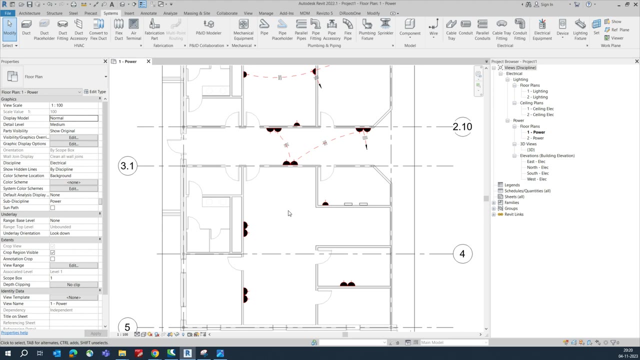 from here and you can give the type of the wire like whichever you need. okay, so just give a dashed and just to give a color like red, okay, and just give a line weight of this one, just click apply. so that will be automatically changing to the here. look like that. so, for example, this to: I need to connect over there. 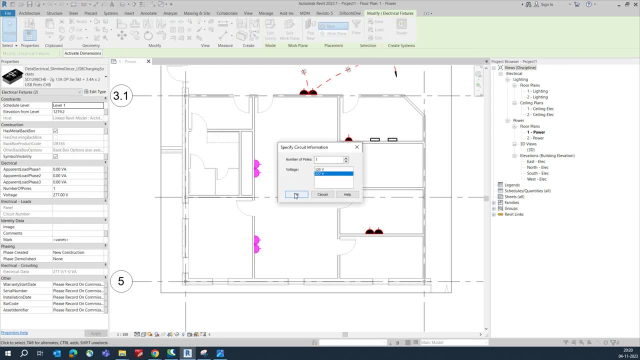 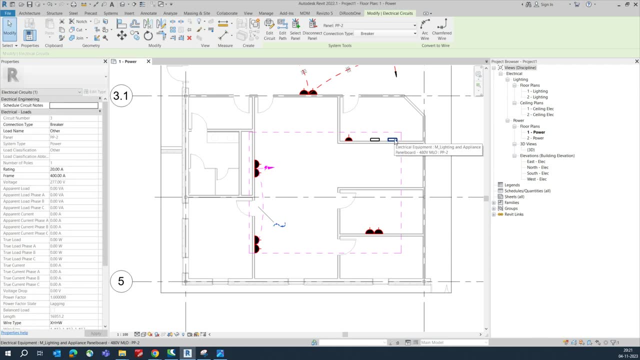 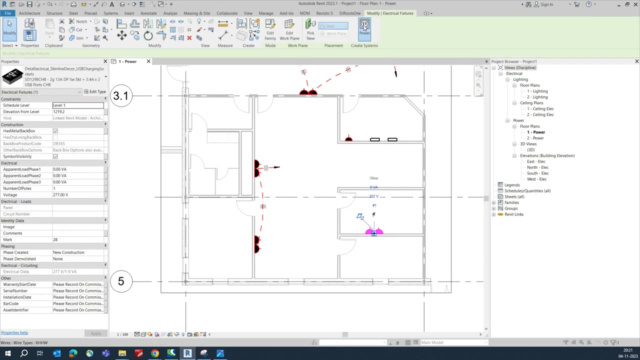 just select that one. select this one, okay, and click this one and select a panel. okay, select a panel- this one I'm selecting- and just give an arc wire so that will be connecting to that panel. okay, same for this one. select this one power. select this one and then click apply and then click apply and then click. 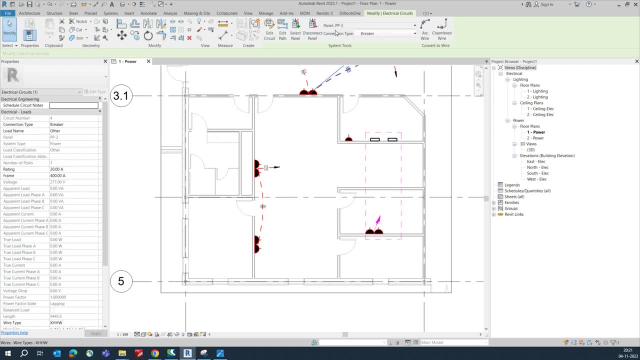 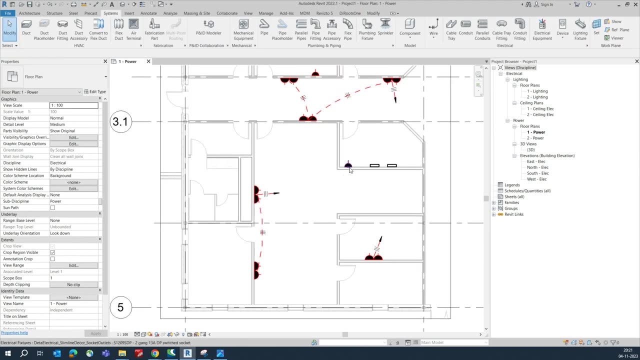 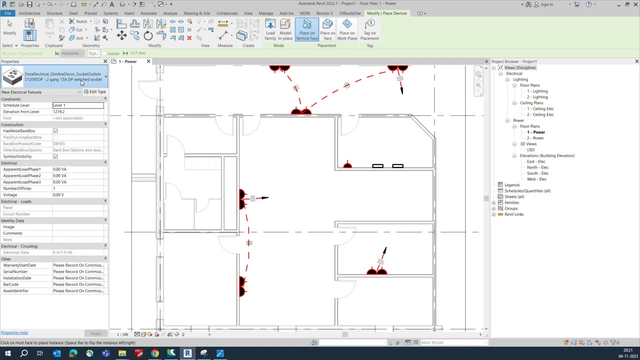 this one, okay, and then I select the panel already selected, then give a arc wire so it will connect it to like this one. so how this socket is placing, you just go to system tab, device, electrical, it fixes. so whichever you need, you can select it from here. so, for example, you need some other sockets, okay, like that. 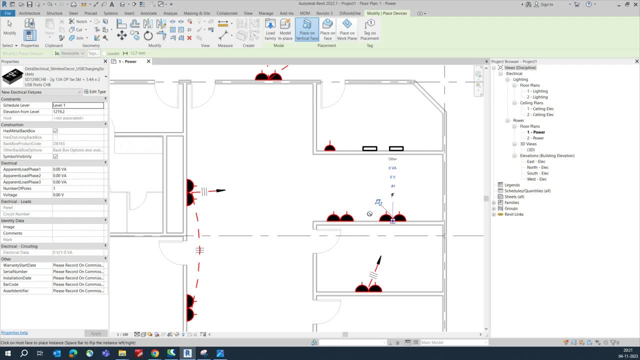 you can. you can easily place this one like this: okay, and even, even as you know, you can easily place this one like this: okay, and even even as you know you can, you can easily place this one like this: okay, and even, even as you know you can. 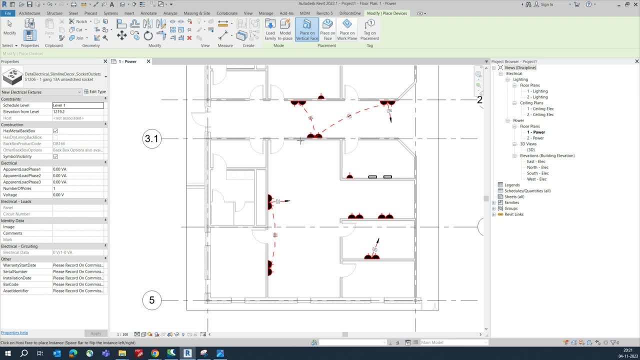 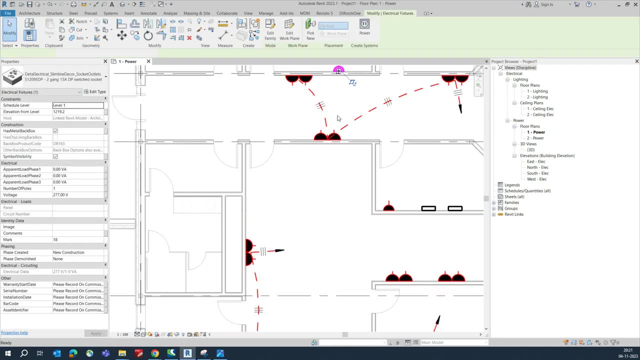 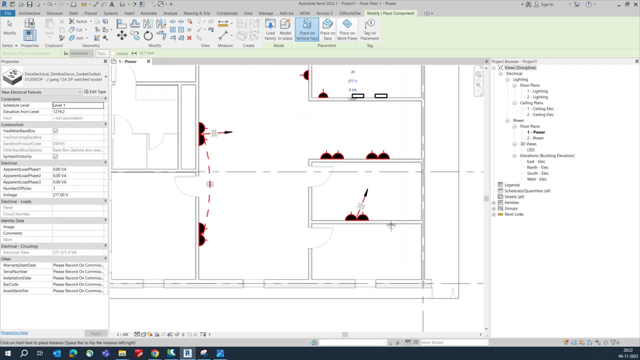 single sockets so you can select the single sockets also. sorry, single sockets, so create similar with this one, okay, just you can place like this, say sockets. you can place like this also: this is not exactly the place, so the placement is you can do like this: okay, so you can give that height of this one also: 450 from. 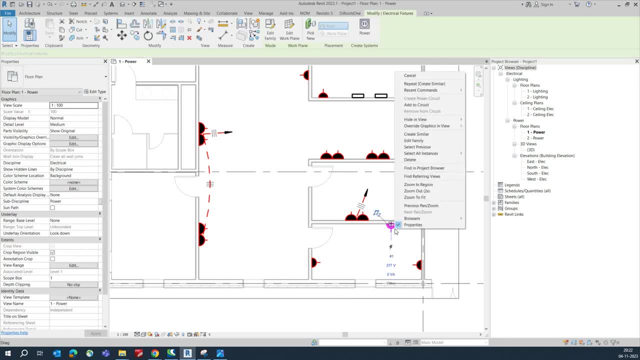 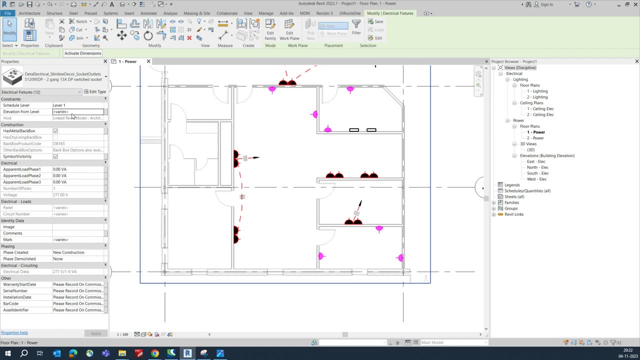 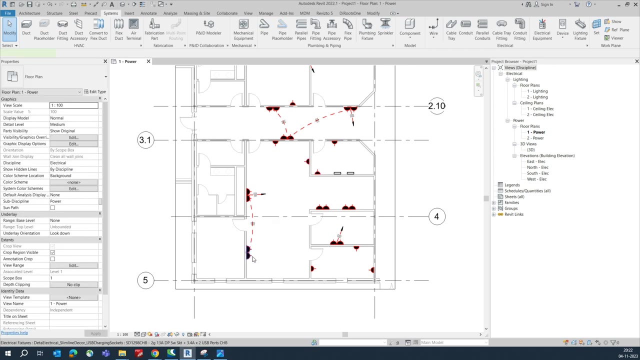 the from the wall, so from the finisher floor level. so you can give like that: select all instance in a visible view. okay, so just will give the elevation 450 from the finisher floor same, like this one also. you can give like that: select, select all instance in the visible view and you just need to give. 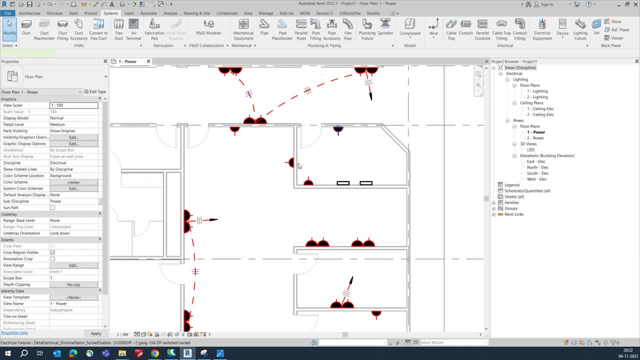 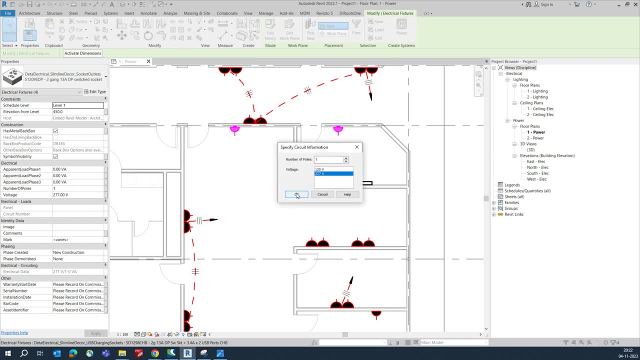 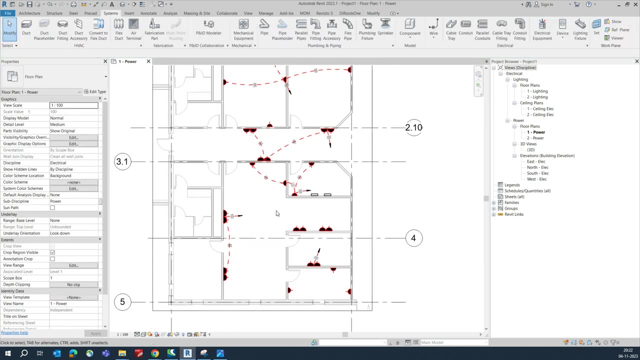 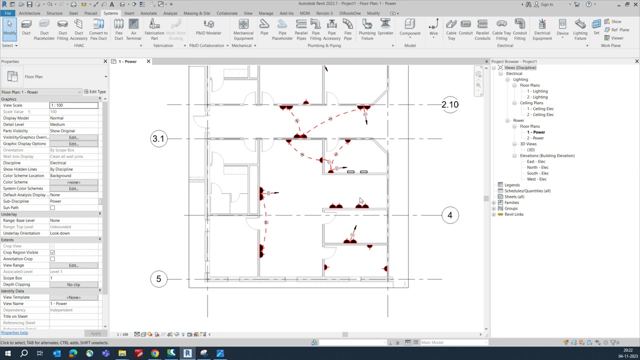 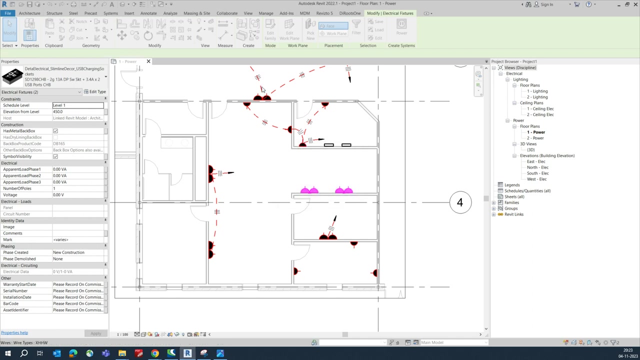 the elevation of this sockets, okay. so if you need to power or giving a power for this three, four for sockets, so select that one power and select this one, okay, and? And then the panel is PP2.. So automatically you can wire that one. So hopefully you guys understood these things, Okay. If you like my video, please don't forget to subscribe. Support me to grow. Okay, Like this power distribution system. you can assign power distribution system simply.